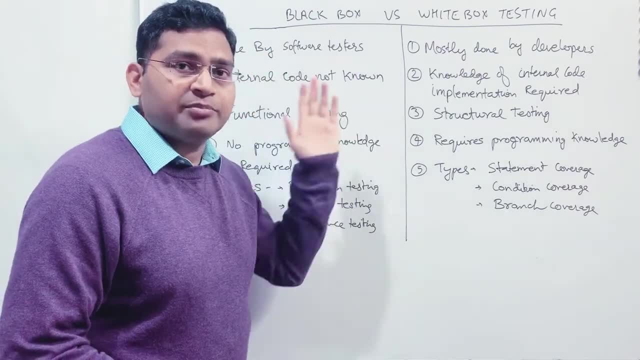 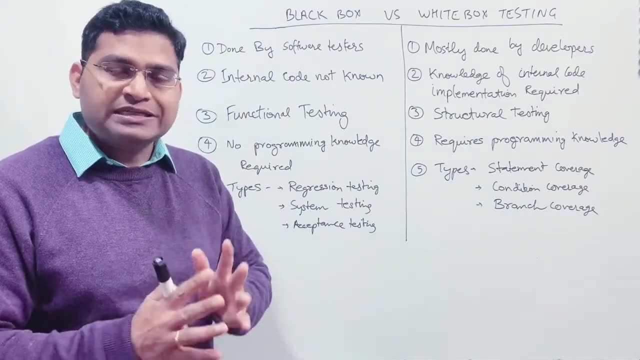 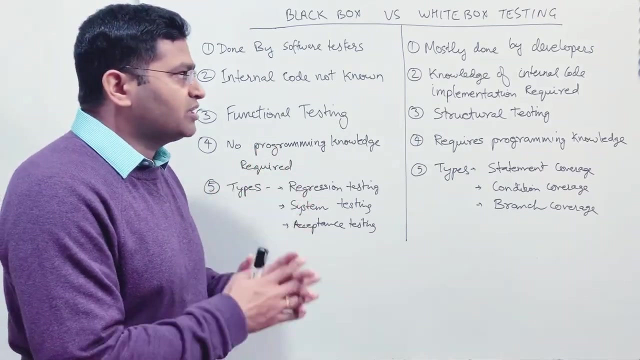 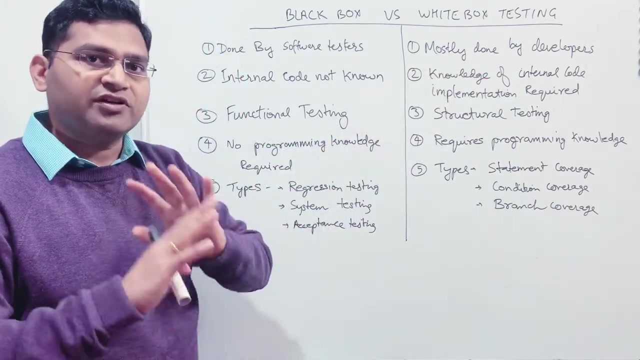 testing, white box testing is mostly done by developers, right. so if, and only if, the tester has the good understanding of the white box testing and programming knowledge, only then the testers do white box testing. but most of the places you will see that white box testing is done by developers. so that's the first key difference, basically in terms of role: who does? 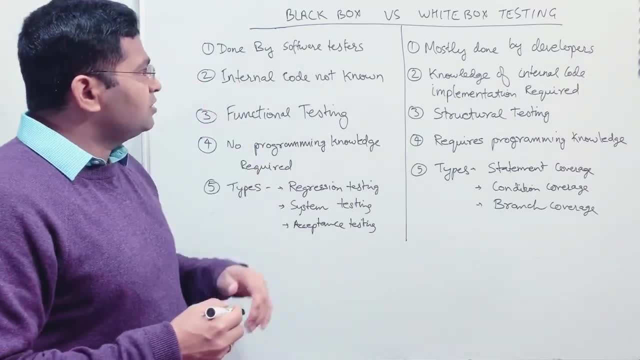 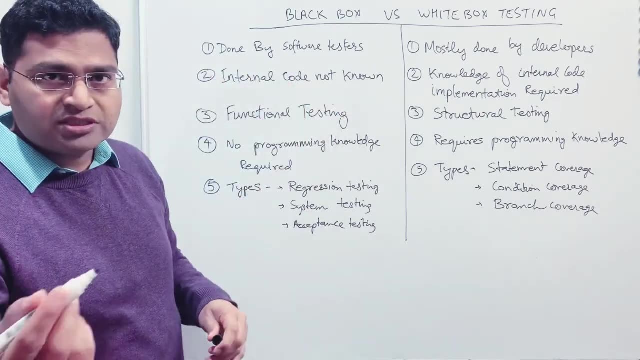 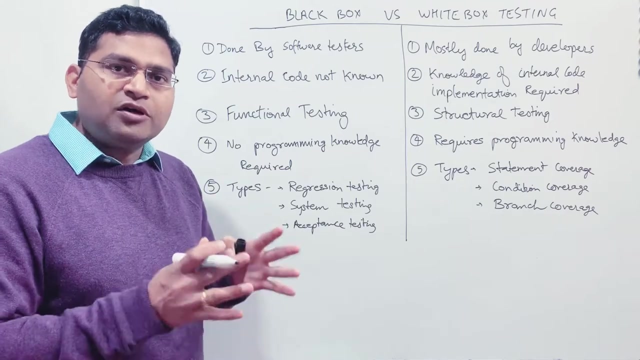 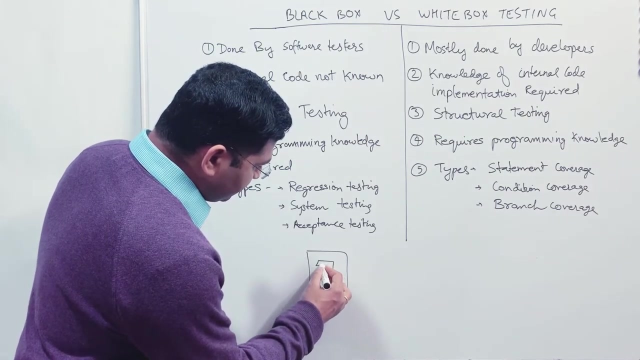 what sort of testing? the second difference is around the what exactly is within the white box or black box testing. so in black box testing, as we have understood you usually as a tester, you usually verify the functionality without worrying about the internal structure of the code, right, say, for example, e-commerce website register link: okay, 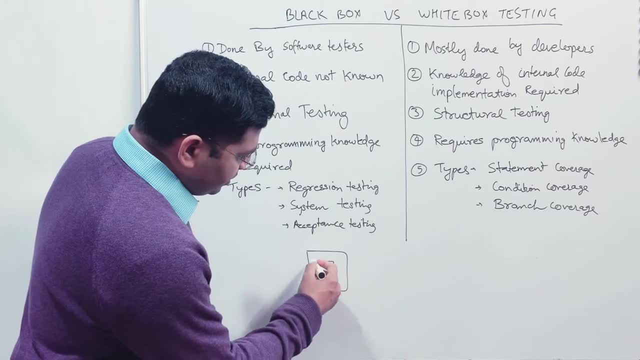 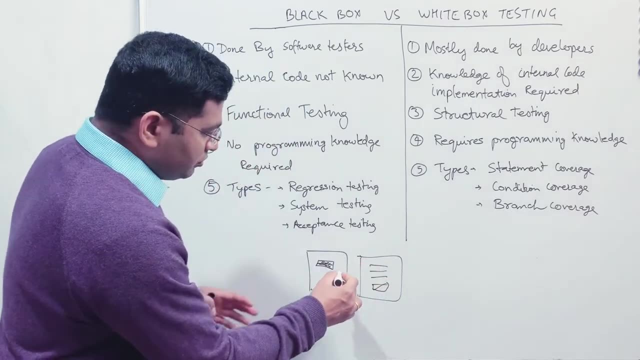 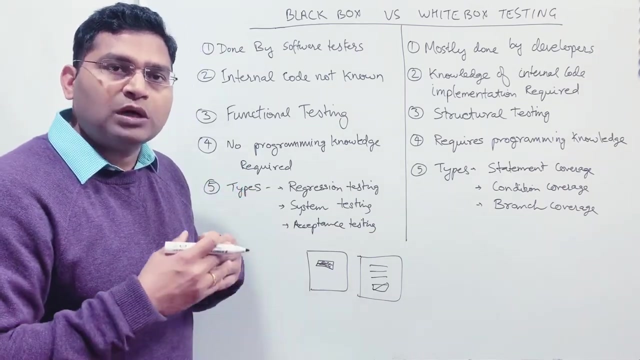 and if i click on a register link then it opens the registration page right and i need to provide all the details there. so once i click on register link, i am not worried about the internal working or how the code has been called. how the request went to server. what processing has been done. 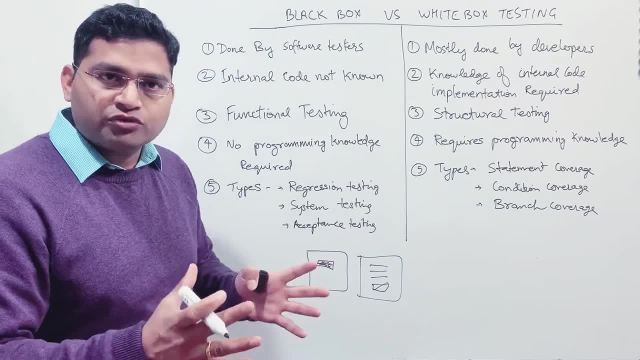 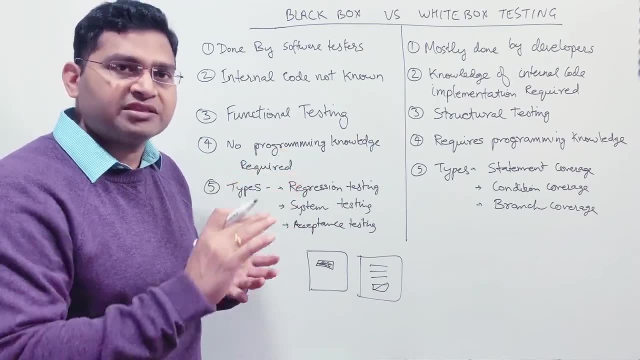 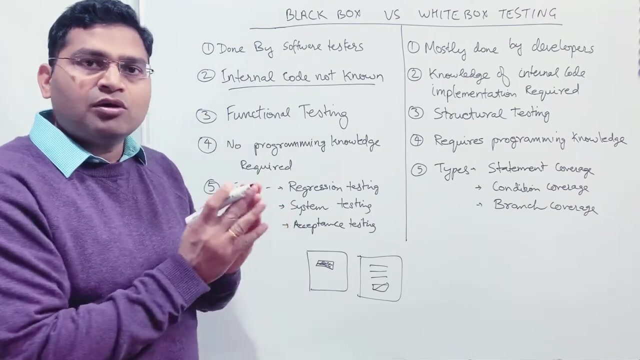 so that is all you know. a black box for me. so once i click on register link, i'm not able to see what exactly happens behind the scene on the server. so internal code is not known in terms of, or in case of, black box testing, or if you are doing black box testing, you don't need to. 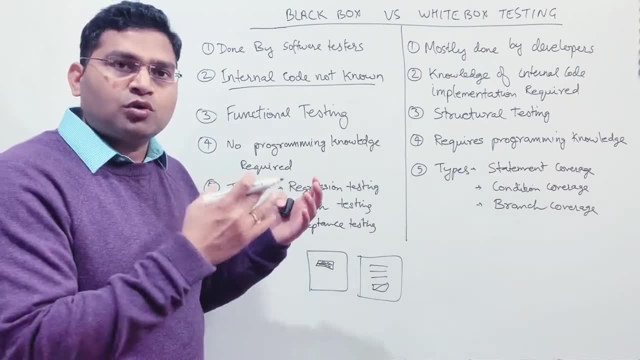 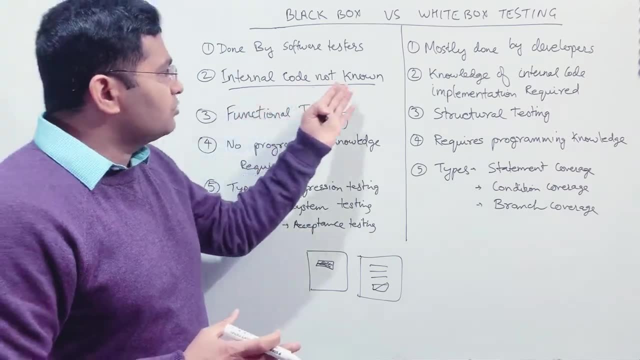 worry about how the internal code is working or what all methods, classes are being written, how the, the overall code is being called internally. so that is not known. if we talk about white box testing, in the same case, knowledge of internal code is not known in terms of black box testing. 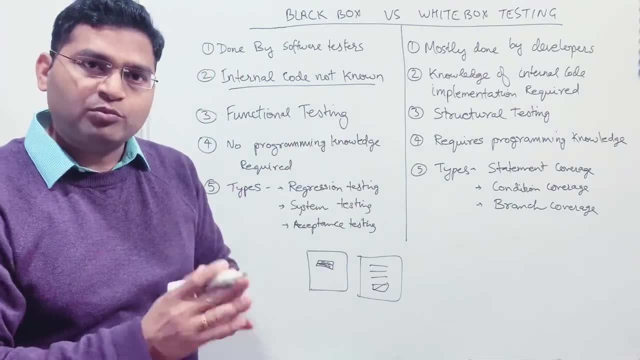 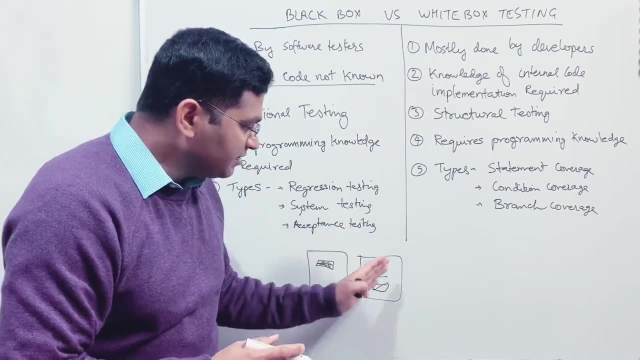 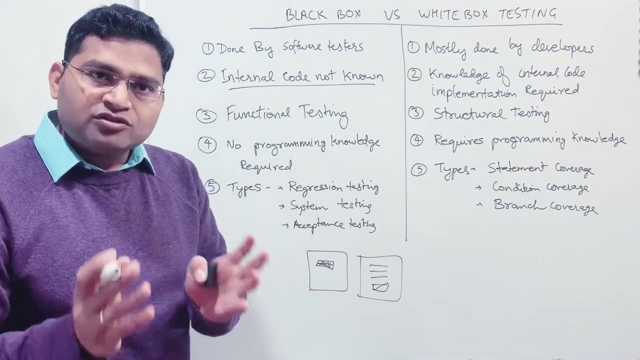 because in the white box testing your testing will not just, you know, not limit to actually clicking on the link and verifying that the page is getting open successfully. in white box testing, the testing will actually be around the coverage of the code that has been written to implement. 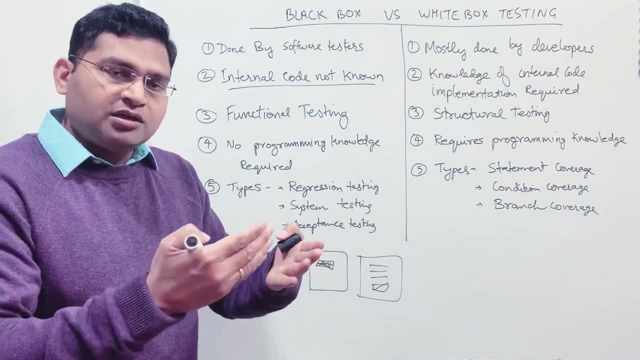 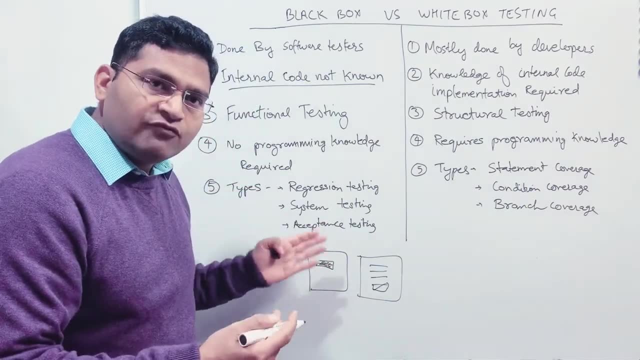 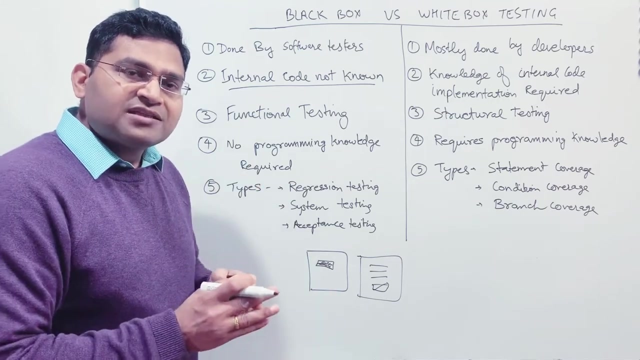 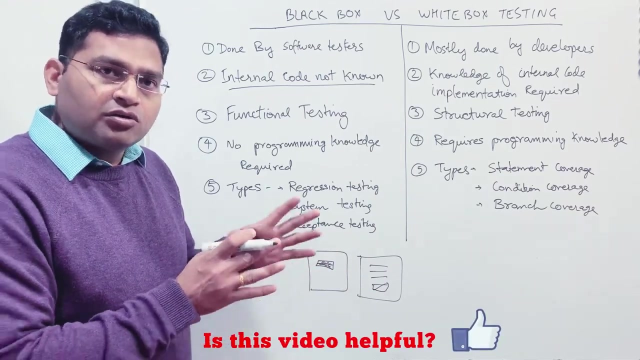 this functionality. so in the white box testing, uh, you will have the. you know, once this particular register link is being invoked, you will verify what all coverage or what all methods are being called and whether, with the test cases, all the permutation combination or basically all the scenarios, statement coverage or the conditions our loop coverage has been. 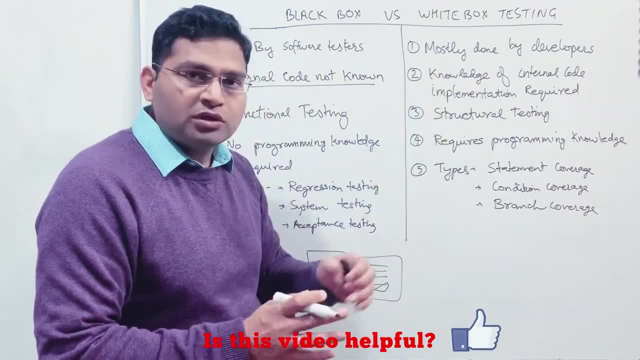 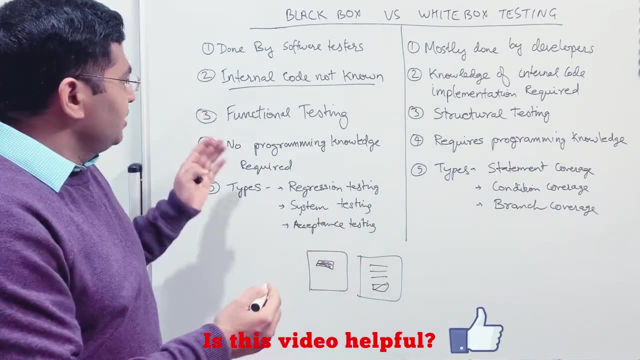 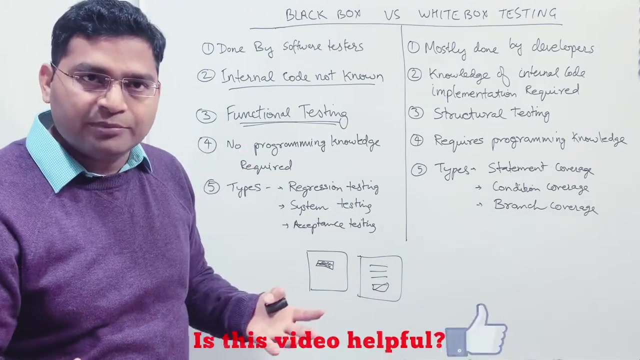 done or not. so that is why knowledge of the internal code implementation is required. if you want to basically verify the internal working of the code, right then. black box testing is the functional testing, right? so verifying the functionality or the requirement: okay. so verifying the functionality, the requirement that is being implemented into. 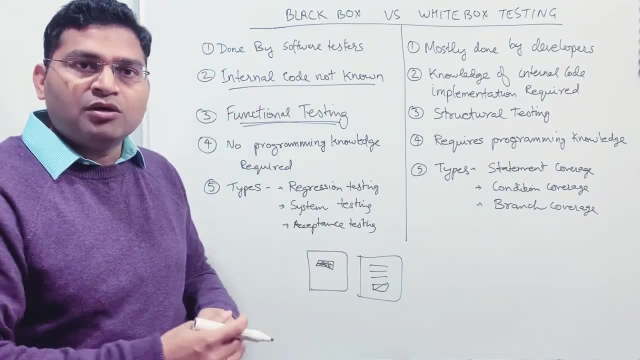 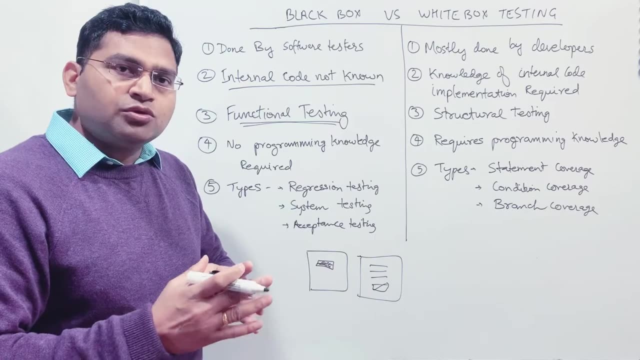 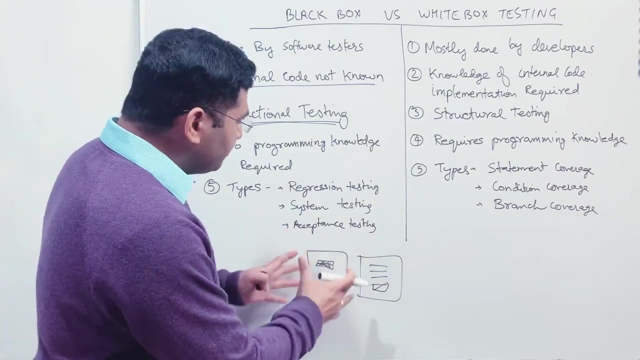 the application. so in this case, registration functionality. or if i am adding the items to the card in the e-commerce website and then checking out, doing the payment. so just verifying the adding items- another functionality. checking out or doing the payment, another functionality. so in the black box, testing, i'm just verifying the functional aspect of the functional testing. 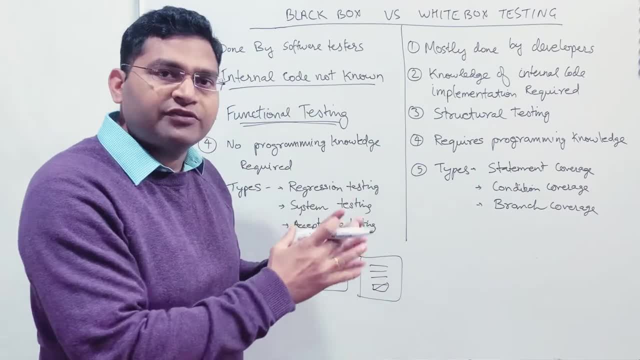 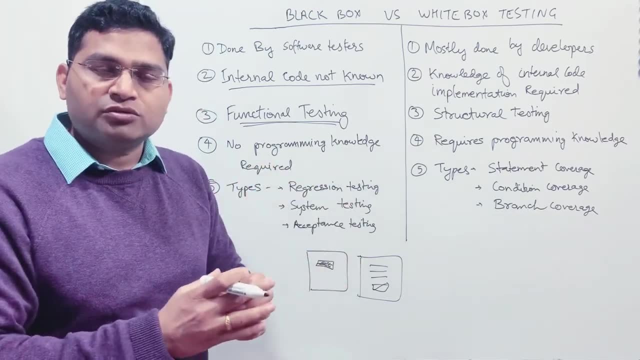 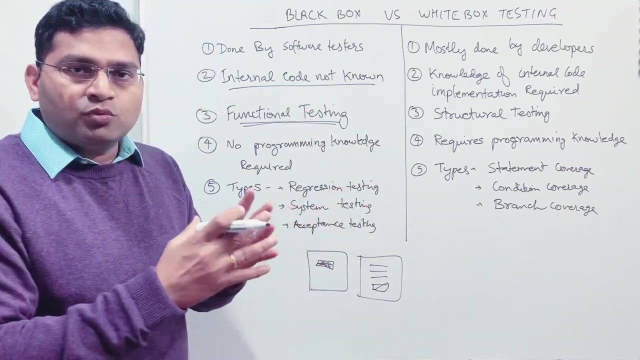 however, in the white box testing, it is structural verification which is mostly for which, which relies on the actual design document. right, so the the design or the low level design that has been done in the project. so when the tech architect does the high level design, hld and the detailed design. 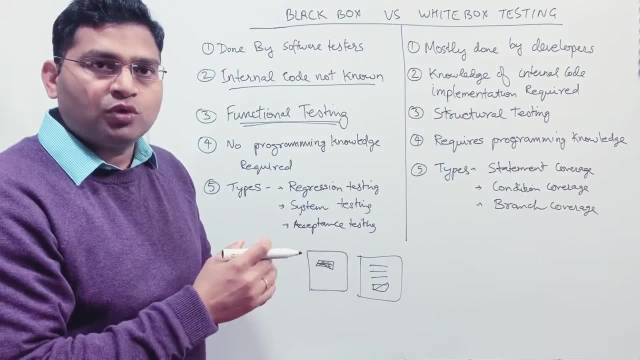 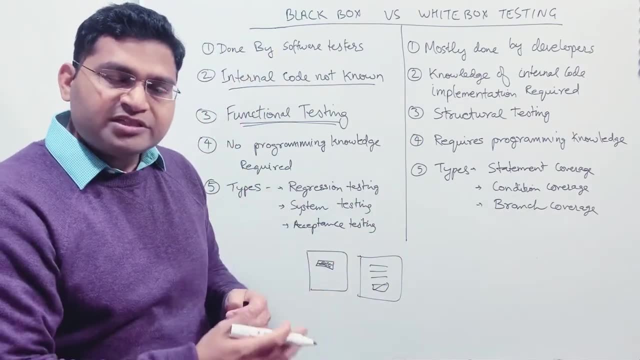 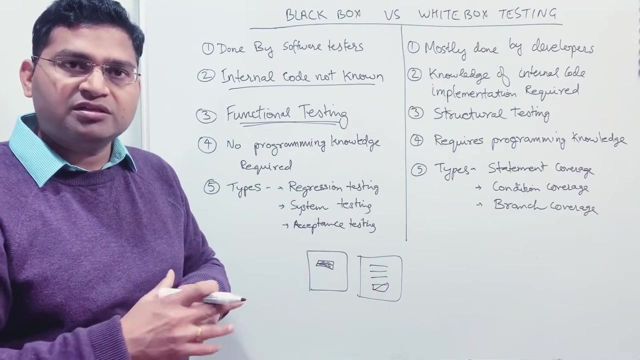 design is required to do the structural testing. based on whatever design has been done, the structure of the code needs to be tested, the statements need to be tested, and how all the aspects or all the methods, classes are being structured and modularized. that all is the purpose of white box testing. so it 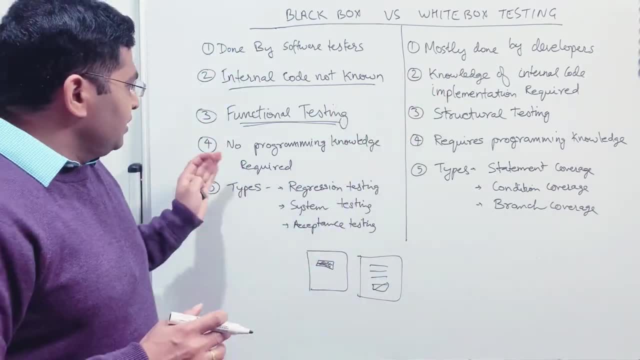 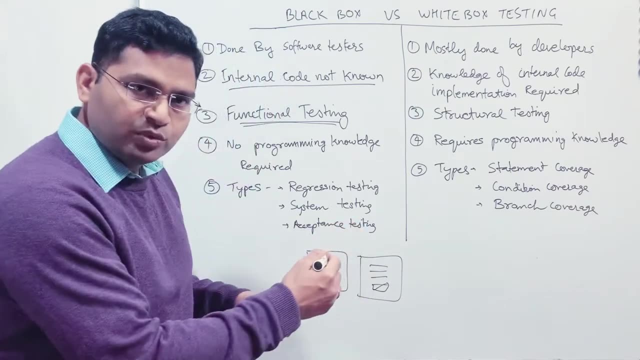 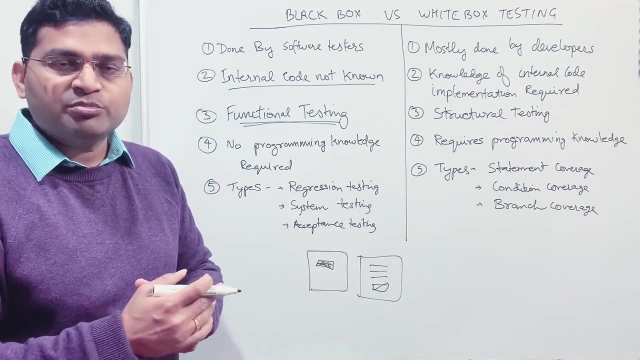 is the structural testing of the software. then in the black box testing, no programming knowledge is required because you don't need to understand what happens internally when you click on register link. you just need to click on register link and you verify the the the web page being opened, the. 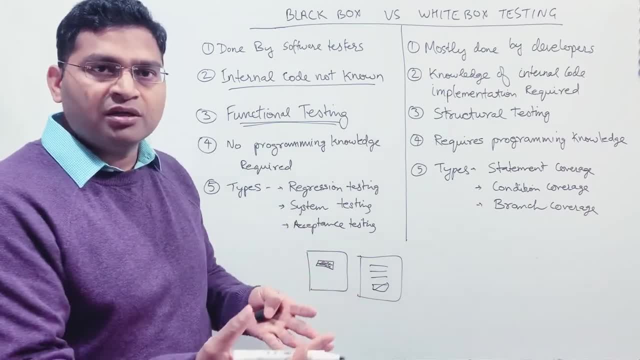 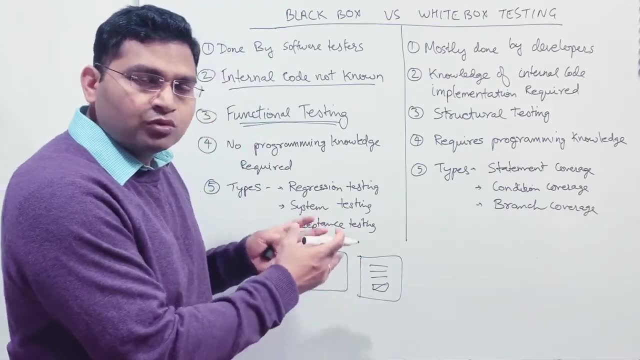 registration page being open right. so that's the verification in the black box testing. so you don't need any programming knowledge or any internal code structure or how the code has been deployed or developed. you don't need any knowledge in black box testing but if it comes, 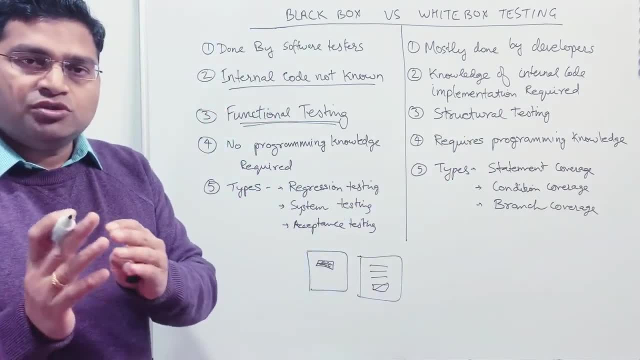 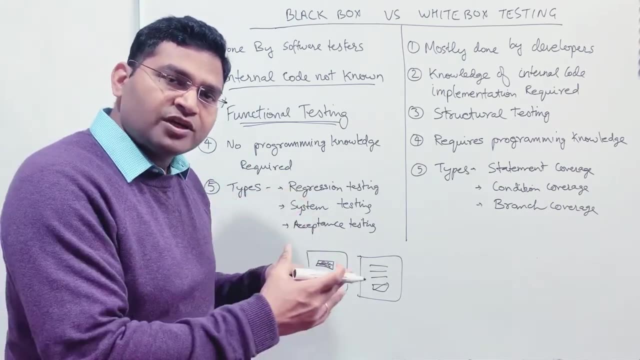 to white box testing. it requires programming knowledge because you need to get into the code. you need to, you know, put the code into different. you know you need to use the testing frameworks to basically write the test cases and then you need to understand the code coverage tools that 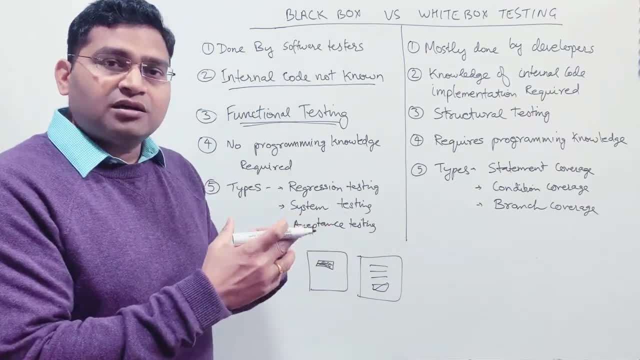 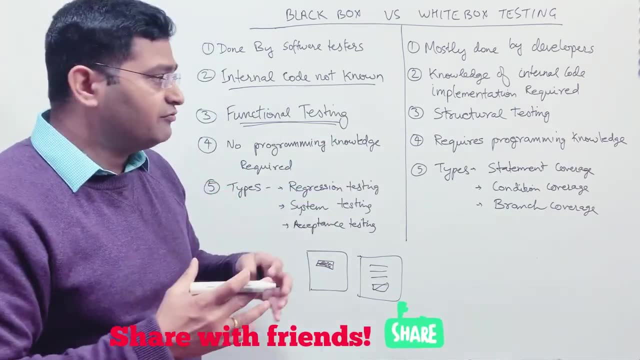 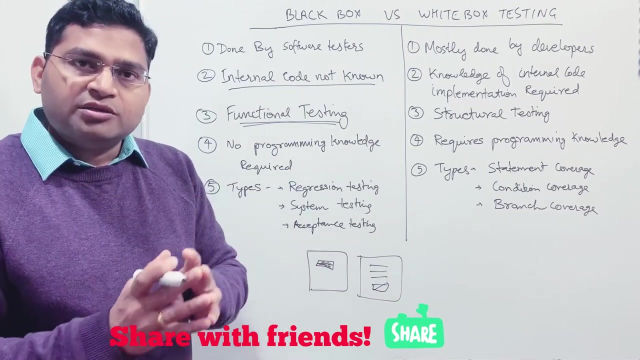 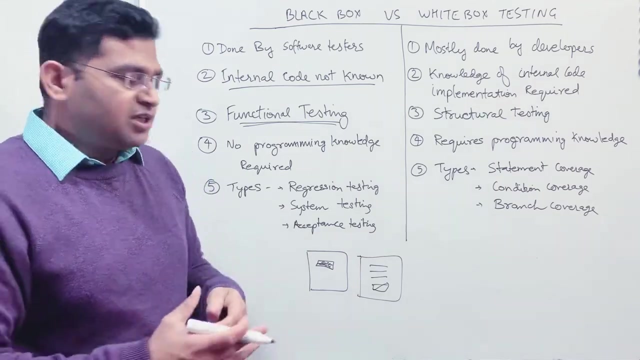 you can utilize and run those testing unit tests or the test cases that you have written in the unit test tools to basically verify the coverage, and because of that, you need to have good understanding of the programming knowledge and the programming in which the particular code or the software has been developed, right? so, if the application has been developed using java, you need. 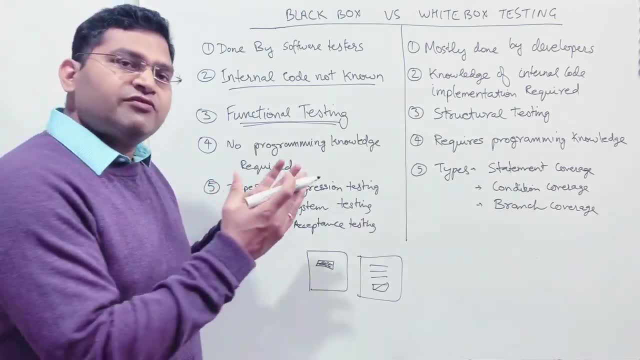 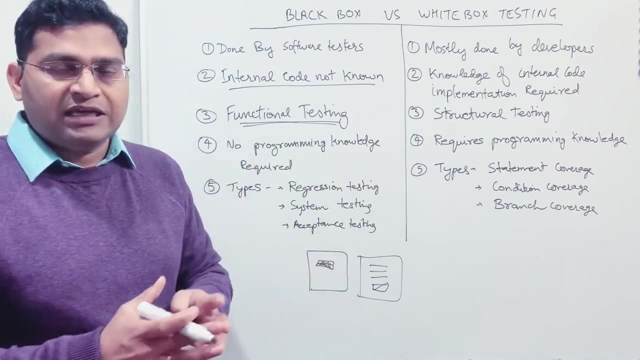 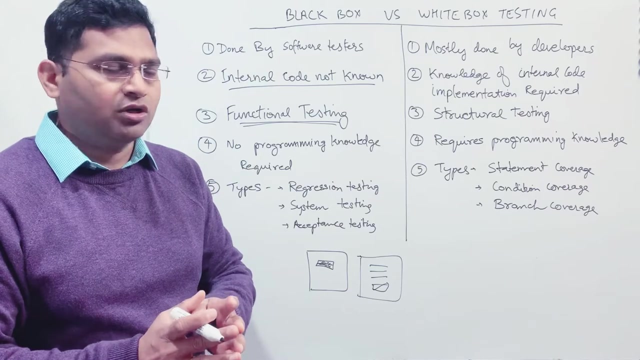 the understanding of java programming language if it is developed using python, you need to understand the python testing frameworks and the understanding of the python programming language right. so that is why in the white box testing you need to have programming knowledge and good programming knowledge to do the white box testing. and that is why the main reason of doing the 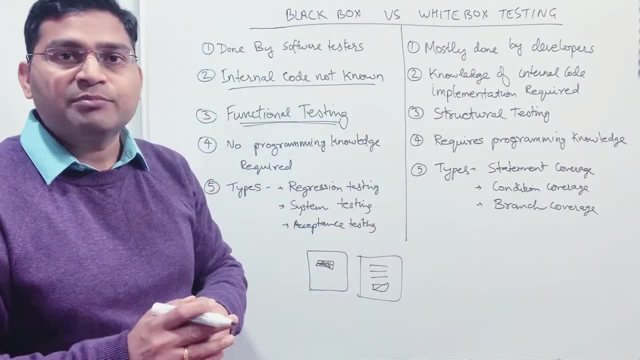 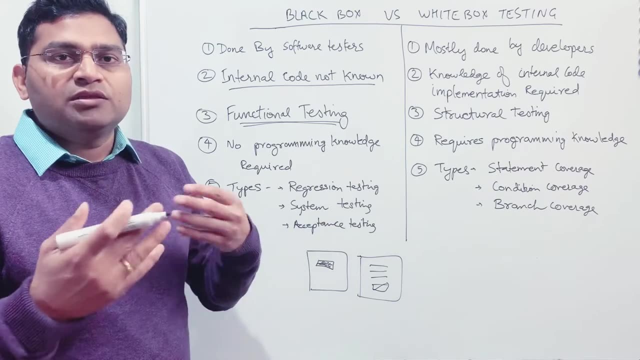 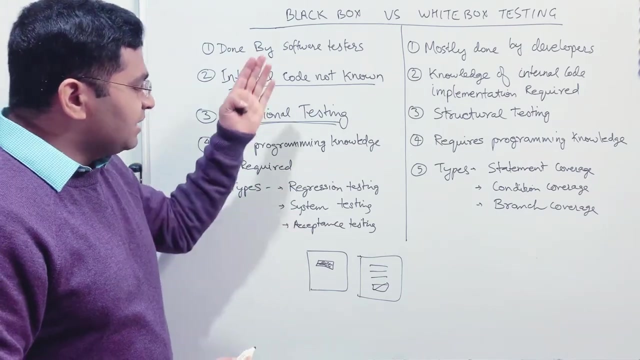 developers, or mostly it is done by developers, because developers have good understanding of the programming language, they have implemented it and that is why they do that particular testing. right then, if we talk about the types, so briefly, i have covered some of the types of black box testing. so regression testing, system acceptance, there are n number of types, so you can, you know. 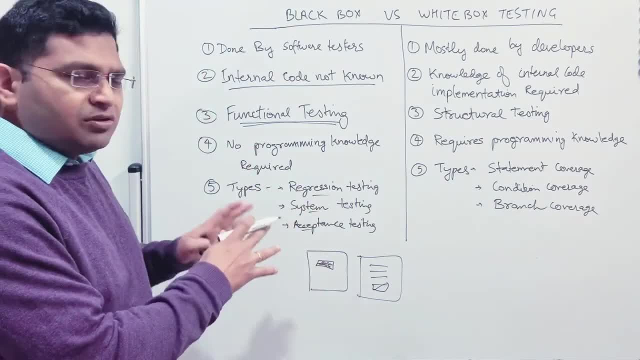 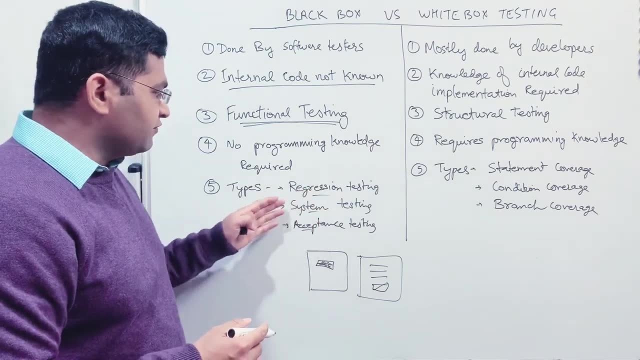 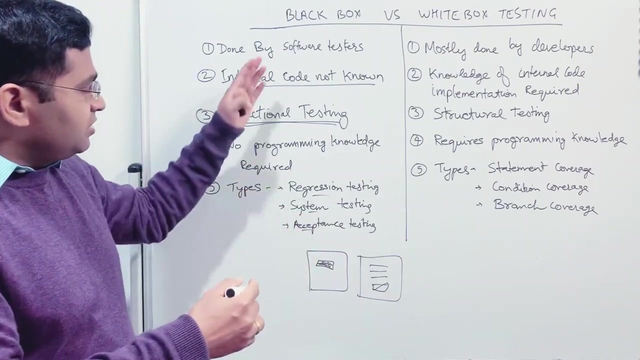 google and search for different types of testing, but in order to you know, go ahead and explain to the interviewer. i think that should be enough. you cover a couple of you know types of testing: regression system, acceptance retesting is another one that you can add. so any other functional. 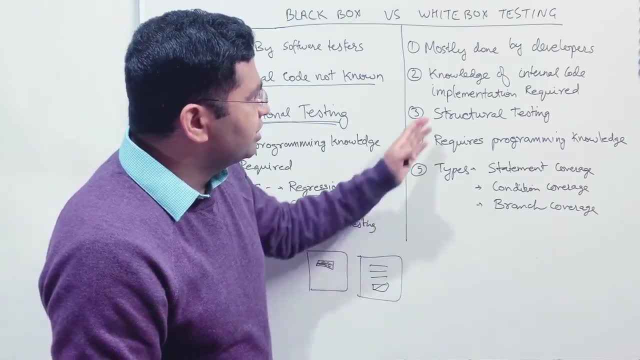 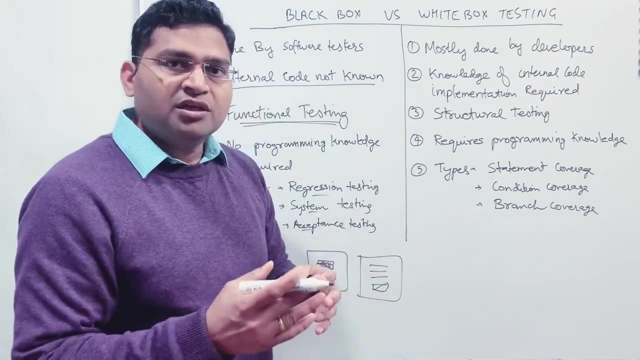 testing that you can think of, you can add in the black box testing. however, in the white box testing the types are: statement coverage, you know you can add in the black box testing, you can add in the, you know, condition coverage, branch coverage. so these are some of the coverage techniques or the